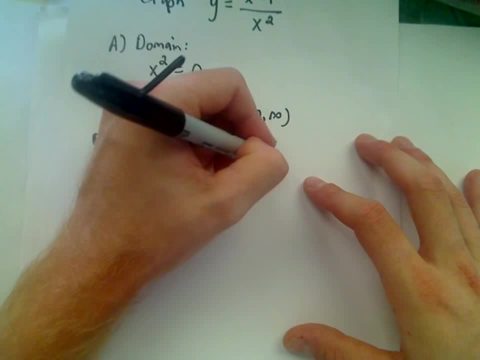 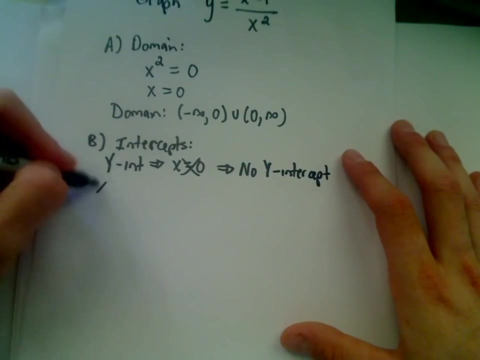 So what that means is: well then, there's no y intercept for this graph. It's just simply not going to cross the y axis. That's okay To find the x intercepts. we set y equal to zero, So then we'll have to solve: zero equals x. 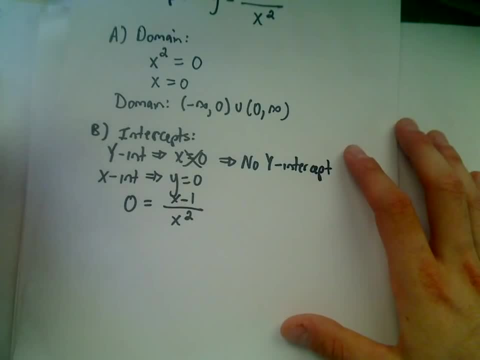 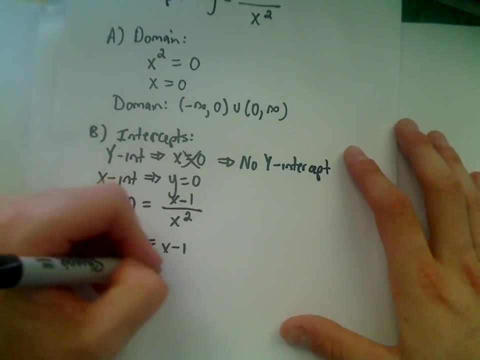 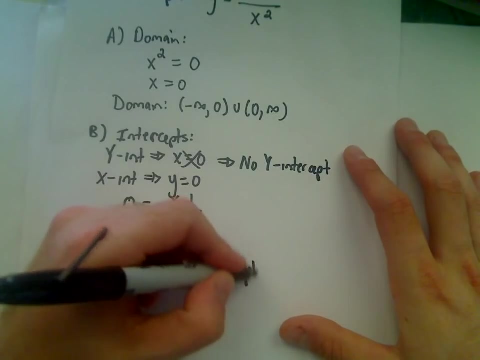 So we'll get x minus one over x squared, And for a fraction to be zero, the top part has to be zero. So really all we have to do is set x minus one equal to zero, And then we'll get x equals one being our x intercept. 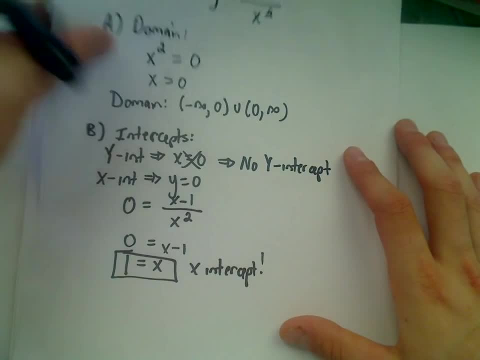 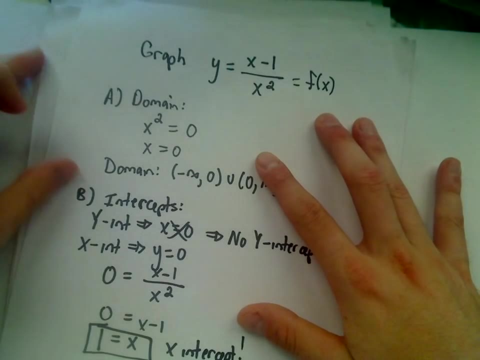 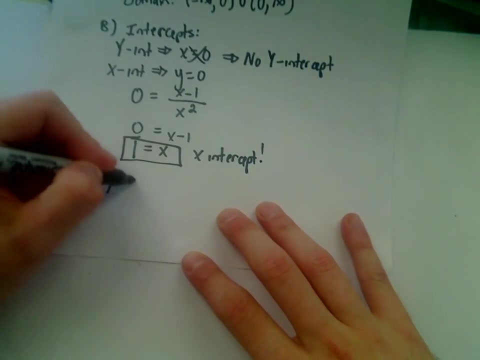 Okay, so we need to keep that guy in mind. Next, let's do symmetry here, So I could label this function instead of y, Let's call it f of x. So remember for symmetry. Let's see if I can squeeze it down here. 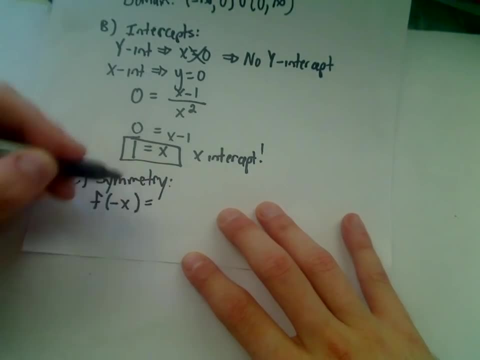 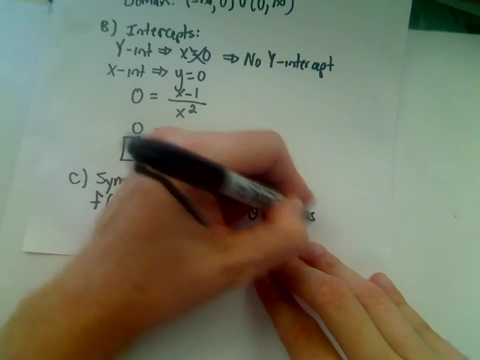 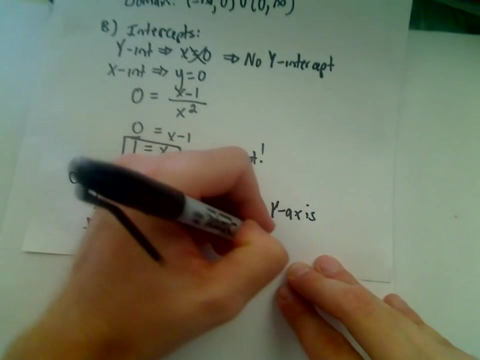 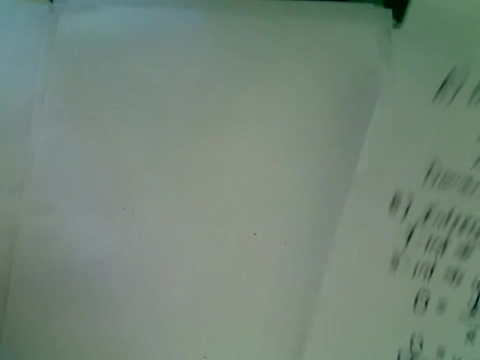 For symmetry. remember: the rule says: if f of negative x equals f of x, it's symmetric about the y axis. And it says: if f of negative x equals negative f of x, then it's symmetric about the origin. So we're going to use this little test just to see whether or not our function is in fact possessing any symmetry. 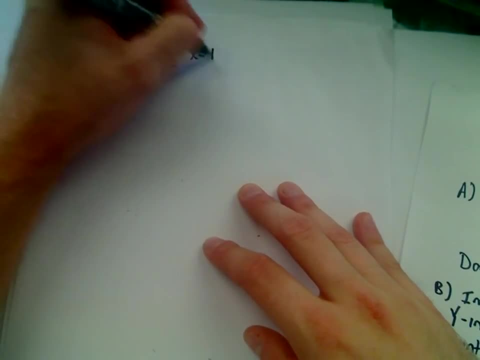 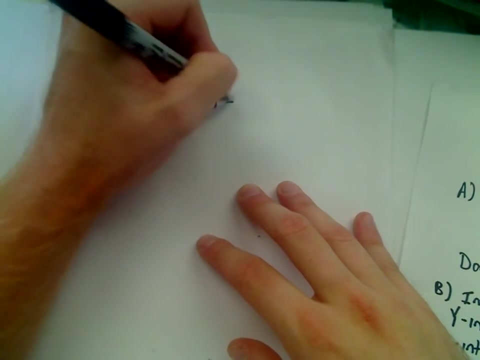 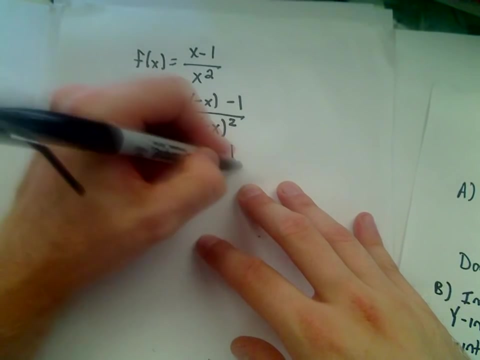 So it says f of x is x minus one over x squared. So if I plug in negative x, I'm going to get negative x minus one over negative x squared, And if you simplify that down, you simply get negative x minus one over x squared. 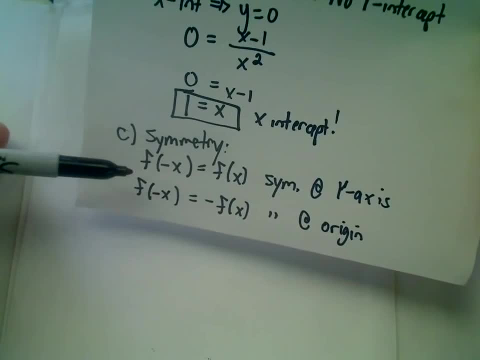 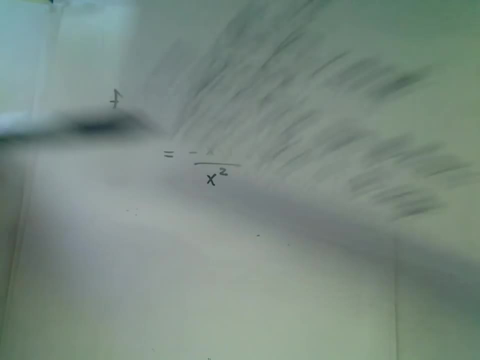 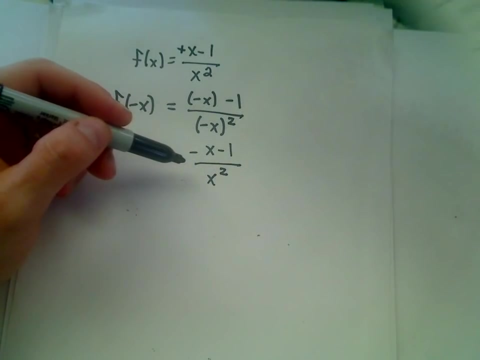 Again, just based on this definition of symmetry. it says if you plug negative x in and you get the exact original out, it's symmetric about the y axis. Well, I don't think we got the exact original thing out because, notice, the original x was a positive and this one's a negative. 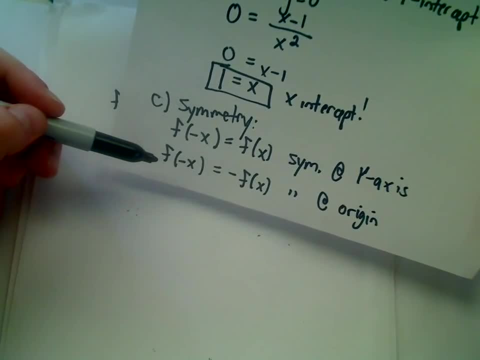 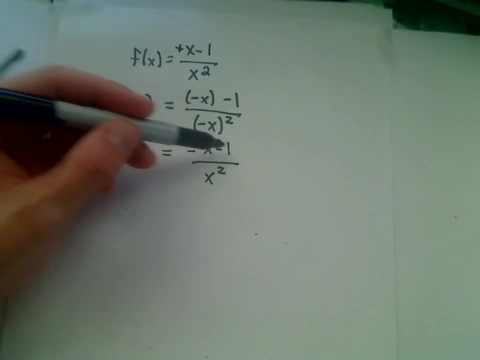 The other condition says basically, if you get the negative of the original, then it's symmetric about the origin, But also it's not the negative of the original. Imagine factoring the negative out of the top. You would get x plus one over x squared. 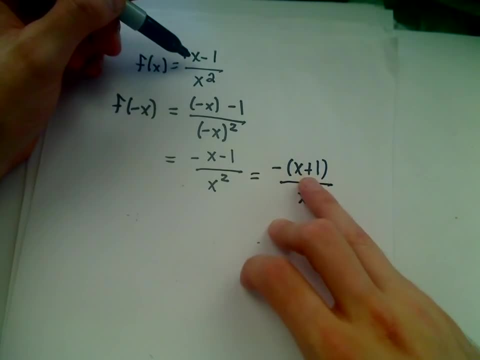 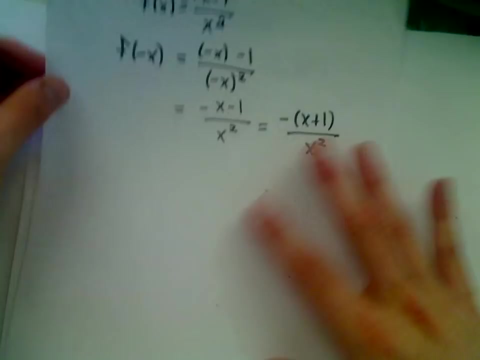 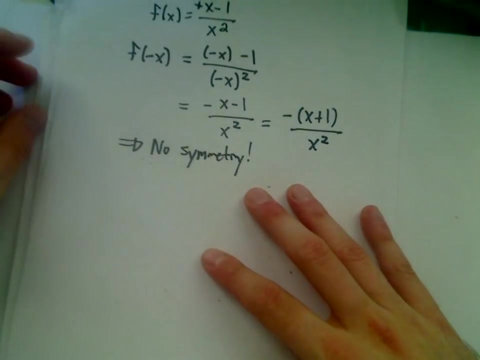 And again, that's not the negative of the original, because the sign on the one is a plus one instead of being a minus one. So the conclusion of the story is that there is simply no symmetry. Okay, so the next thing we'll do is we'll talk about asymptotes. 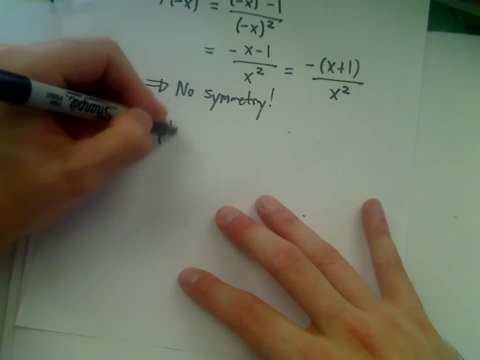 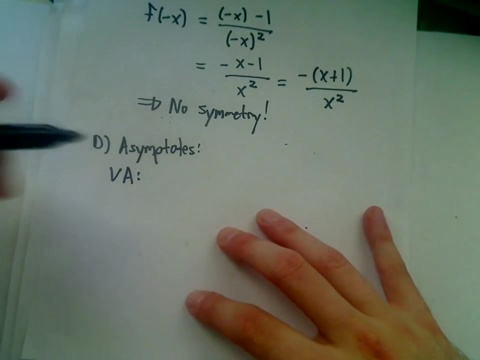 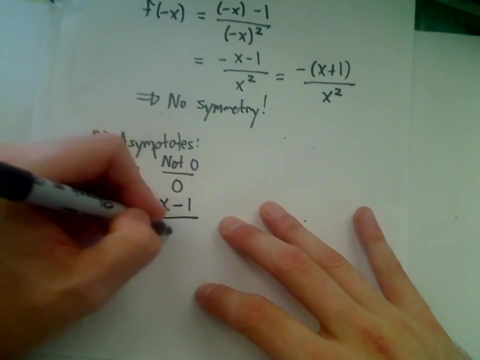 And remember, for rational functions you're going to get a vertical asymptote, basically, where the denominator is zero but the top simultaneously has to be not zero. Okay, so if you look at our again our function, we already said that x equals zero, makes the denominator zero. 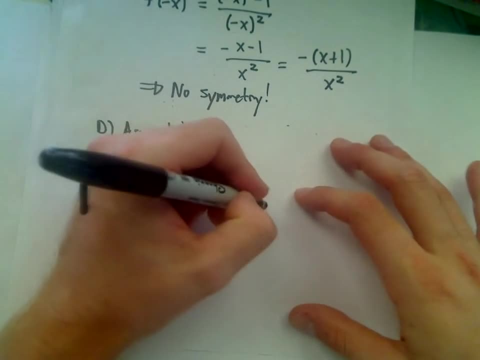 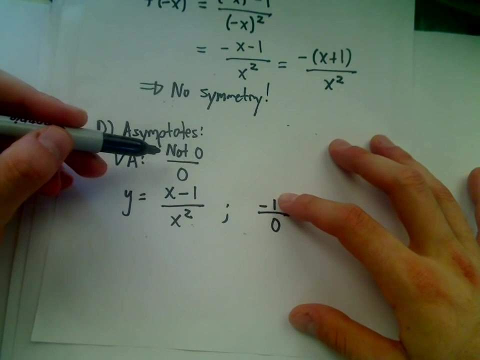 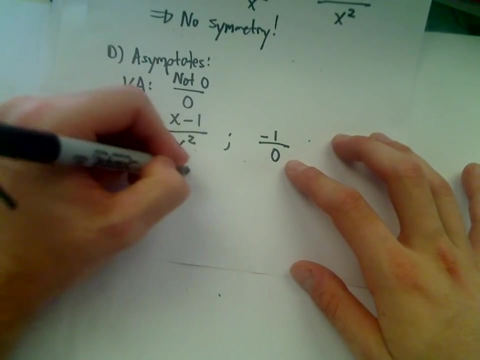 Well, it certainly doesn't make the numerator zero. Imagine plugging in zero. You get negative one over zero. Again, we're getting this little property that we have: a number that's not zero divided by zero. For rational functions that implies that the line x equals zero, is a vertical asymptote. 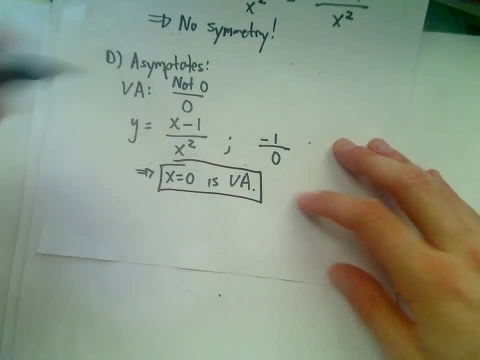 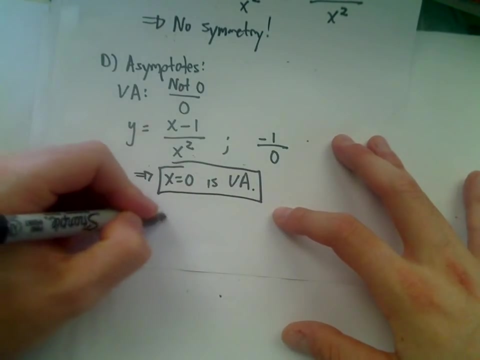 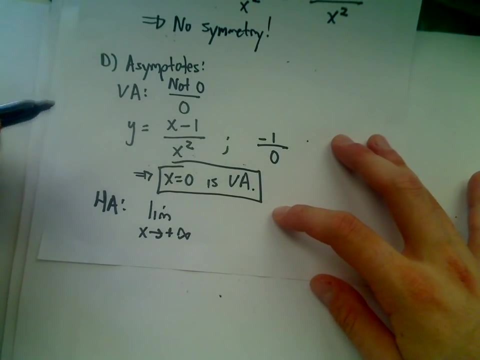 The next thing we would have to do is find a horizontal, any horizontal asymptotes, And remember to find horizontal asymptotes. You look at the limit as x goes to positive infinity, and then you also look at the limit as x goes to negative infinity. 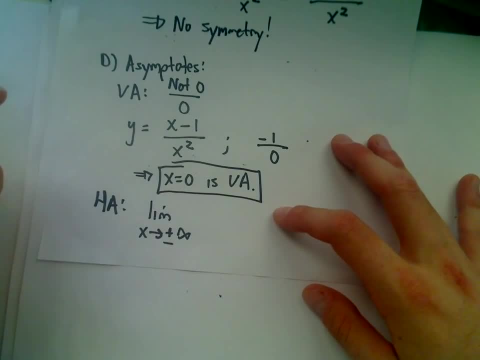 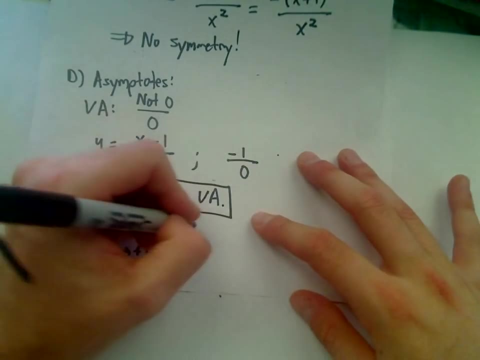 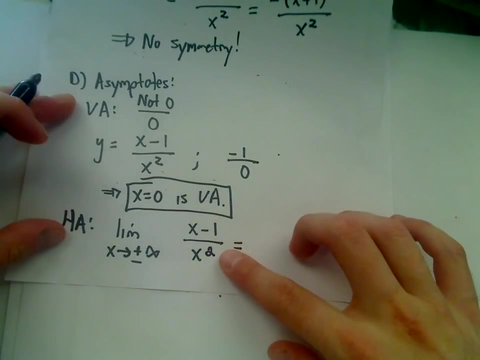 But again for rational functions, it turns out you can do them simultaneously. Whatever, if the limit on one side exists, the limit on the other will exist and it will be the same number. There's a trick for rational functions. It says: if the power on bottom 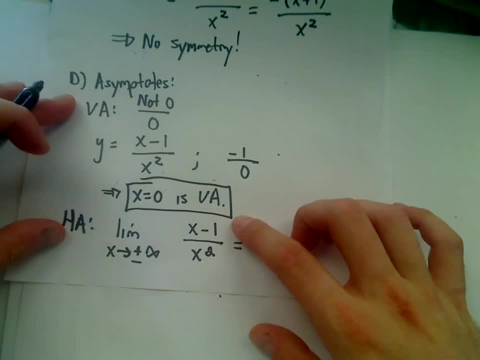 if the degree of the polynomial on the bottom is bigger than the degree of the polynomial on top. in the denominator we have a polynomial of degree two. On the top we have a polynomial of degree one. It says that this limit will always work out to be zero. 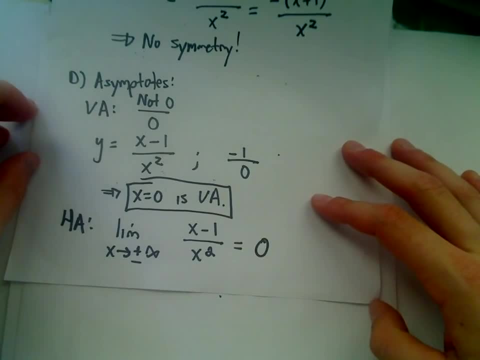 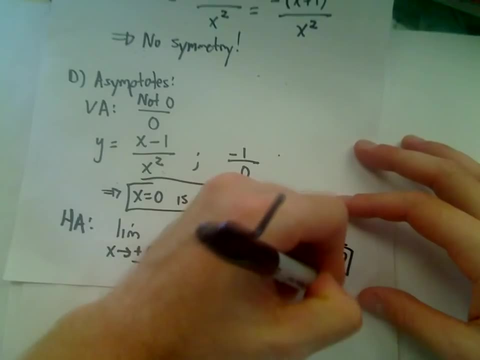 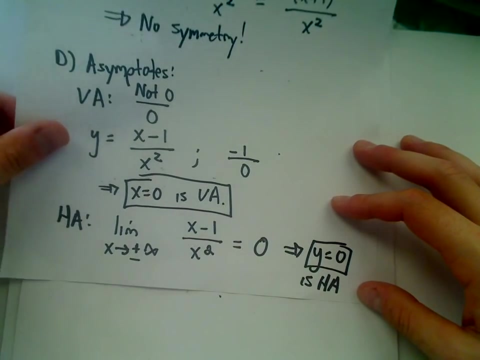 And I do these in another video talking about limits at infinity and, I believe, for rational functions. even So, this says that the line y equals zero is going to be a horizontal asymptote, So we'll have to use that When we sketch our graph, obviously. 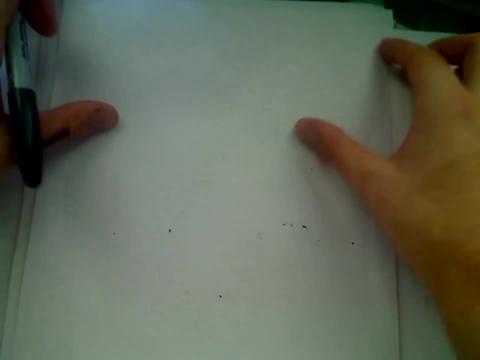 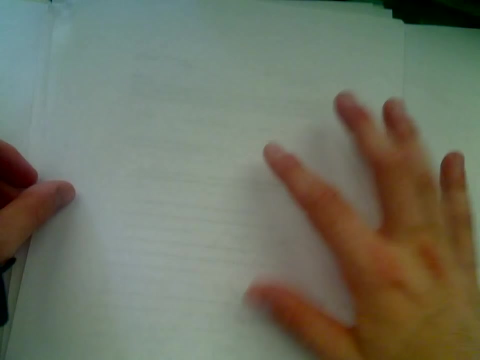 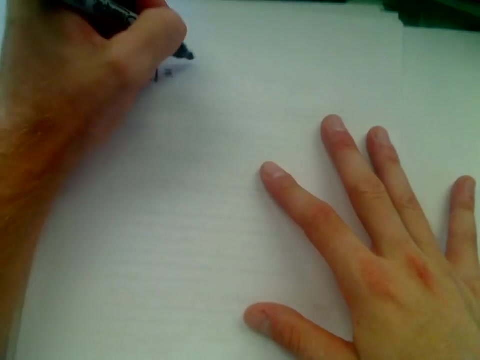 The next thing we need to figure out are intervals of increase and decrease. So to find intervals of increase and decrease we're going to have to take the derivative of our function and figure out. do our little sign chart and figure out again where the derivative is positive. 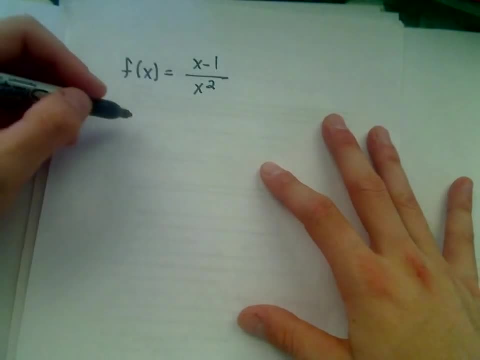 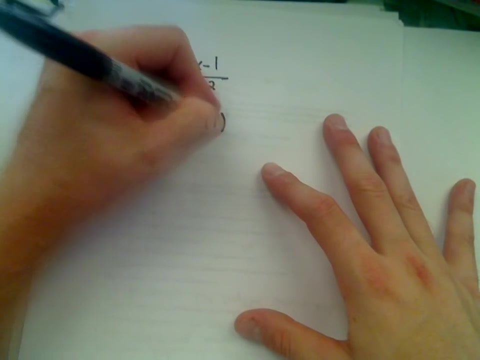 and where the derivative is negative. So it looks to me like if we take the derivative, we're going to have to use the quotient rule. So the quotient rule says you get the bottom times the derivative of the top, which will just be one. 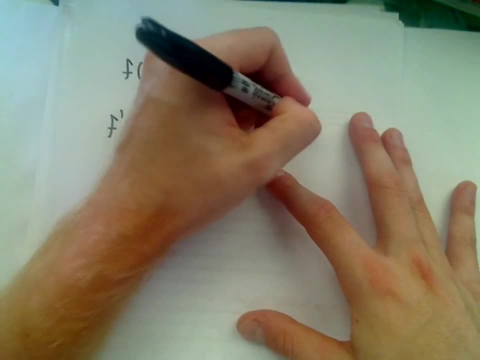 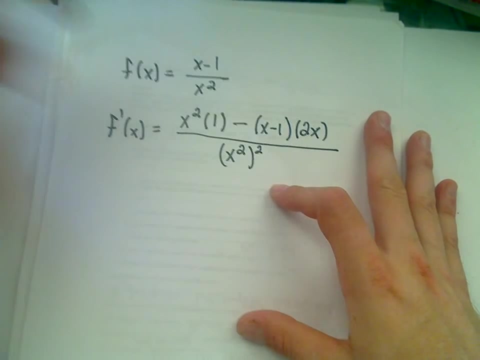 minus the top- make sure you put that in parentheses- times the derivative of the bottom, which will be 2x all over the denominator squared. Okay, so we need to clean this up a little bit. It looks like in the numerator you get x squared. 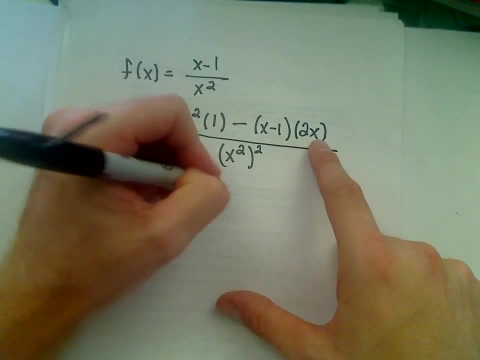 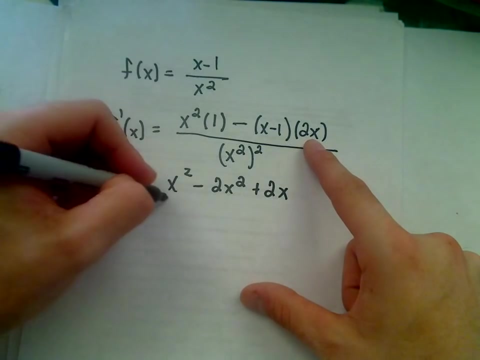 We'll get x times 2x, which is 2x squared, but we have to distribute the negative. so we'll get negative 2x squared. Negative one times 2x is negative 2x, but again we'll have to distribute the negative. 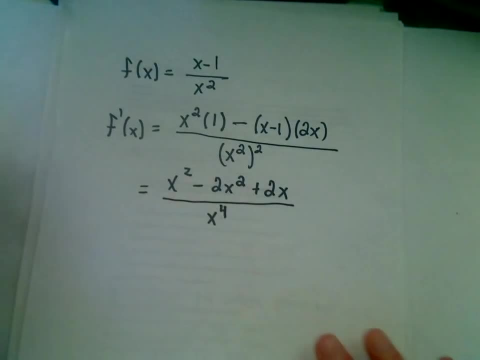 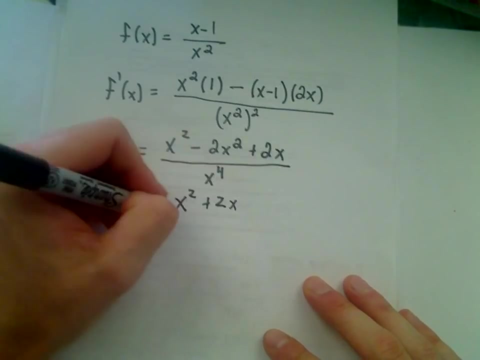 and make it positive 2x, We get x to the fourth. on the bottom, If we combine our like terms, it looks like we get negative x squared plus 2x over x to the fourth. So now all I'm going to do simply is factor an x. 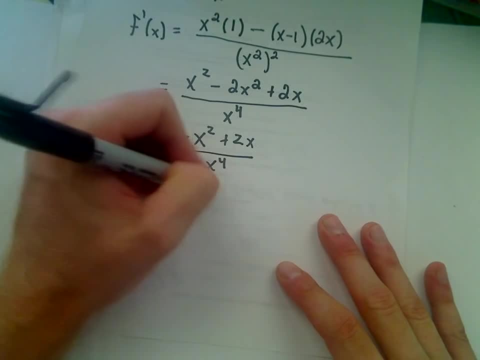 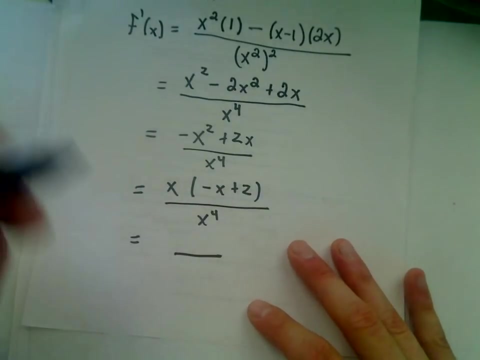 out of the numerator just to clean things up, and it looks like we'll have negative x plus 2 over x to the fourth. My x on top will cancel out with one of the x's on the bottom, leaving me with just x cubed. 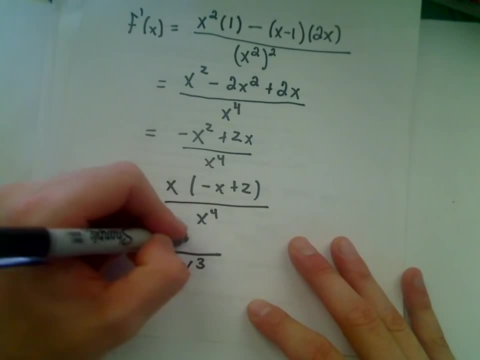 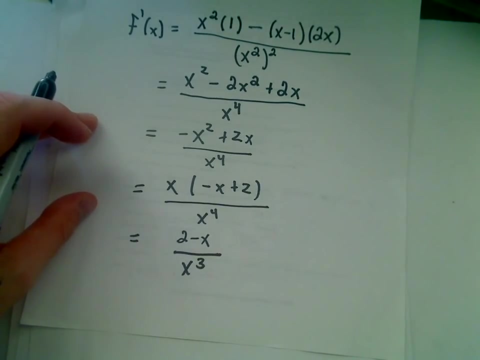 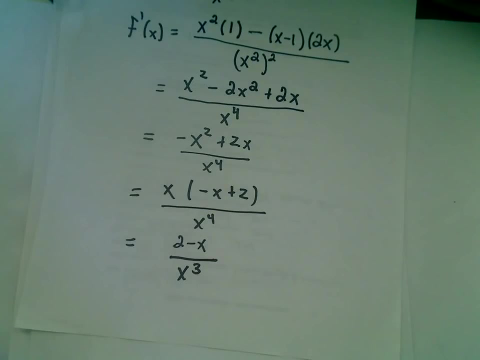 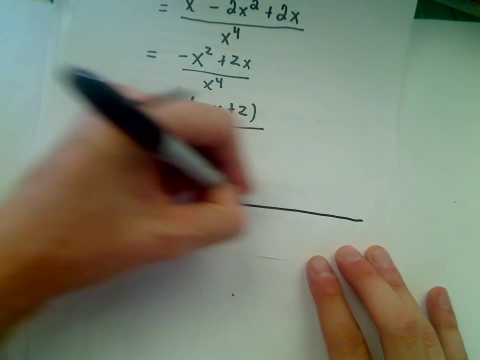 and I'm going to rewrite that thing now as just 2 minus x, just because I want to. I think it looks a touch better that way. So at this point we have to make our little sign chart. Remember, we have to find the critical numbers. 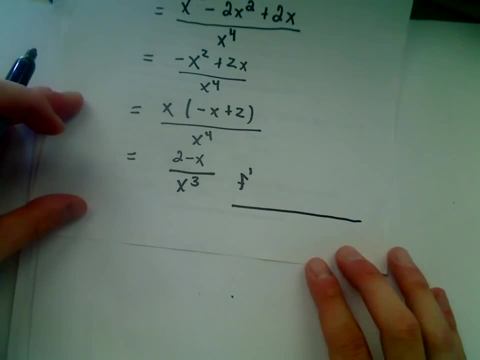 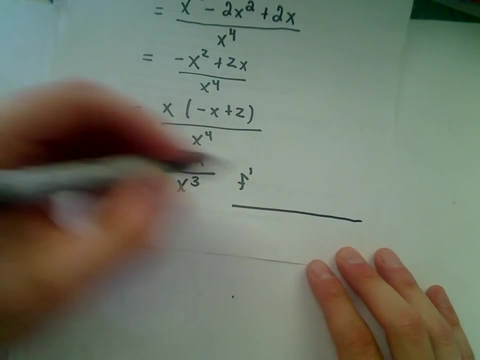 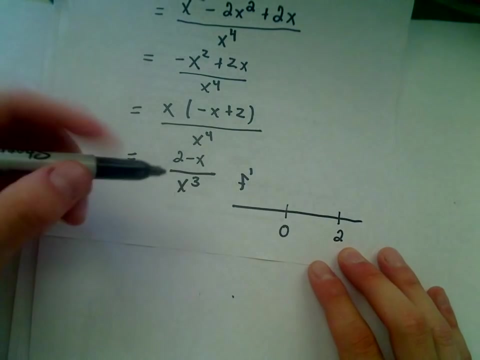 of the denominator, The first derivative. Technically, you just want to look basically where the first derivative is undefined and where it equals 0. Well, it's going to be undefined when the denominator is 0, which is 0. The numerator is going to equal 0 when x equals 2..